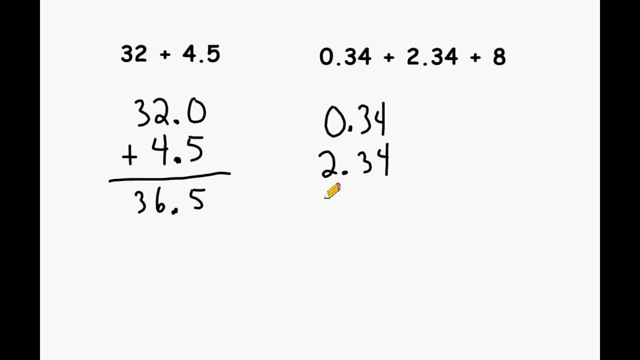 is 8 and the last value is 8. We have to write that in the ones column. And we may add a decimal right after the number 8 and add zeros to hold these place values for us. And we add these values together and we may start by dropping our decimals straight down. 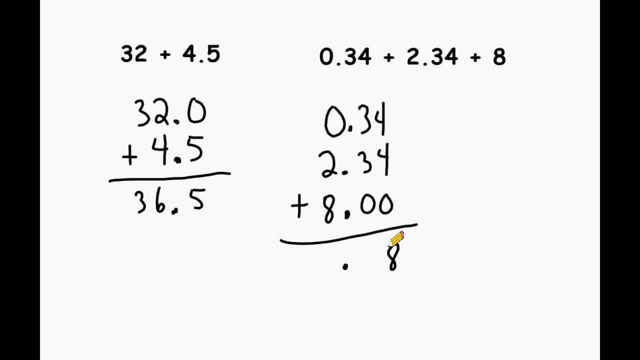 In the hundredths column we have a total of 8 hundredths. In the tenths column we have a total of 6 tenths. And in the ones column we have a total of 10. So all three of these values added together 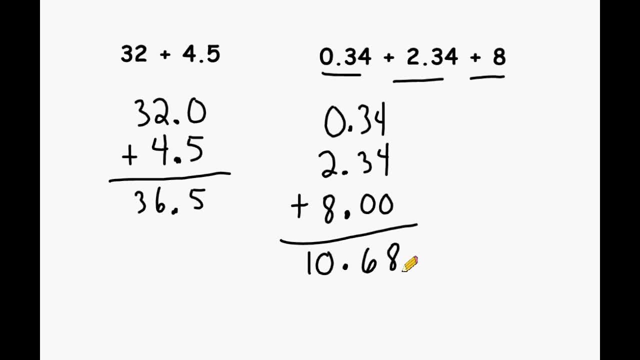 yields a sum of 10 and 68 hundredths. Now let's try some subtraction. 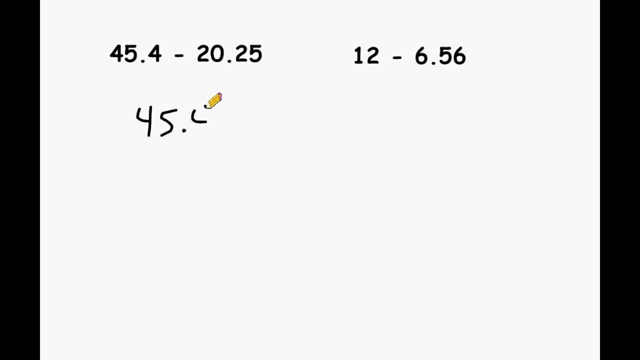 We have 45 and 4 tenths. And from that we are going to subtract 20 and 25 hundredths. And four plus 4 will be 95. Then we subtract 10 minus 10 to turn 오� branding matrix into plus 10. And now we have the remaining sum of 45 and כ. 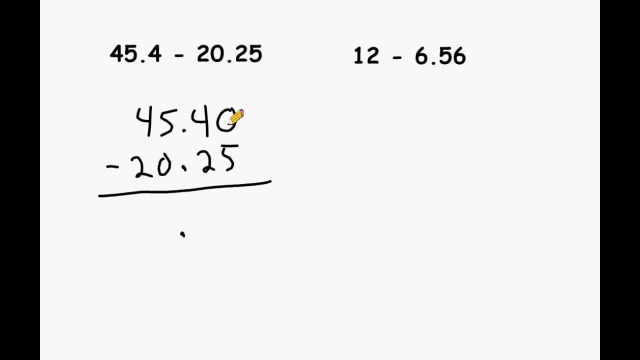 And we can write these which are the result. And we don't have to counted this in the Mysteries for now. We can do a moment only. 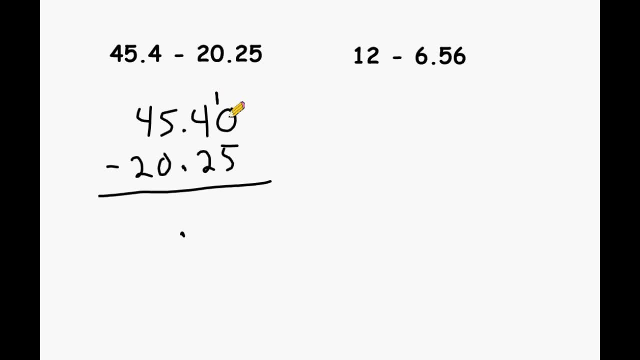 All product functions able to write form applications are provided in a field of code. 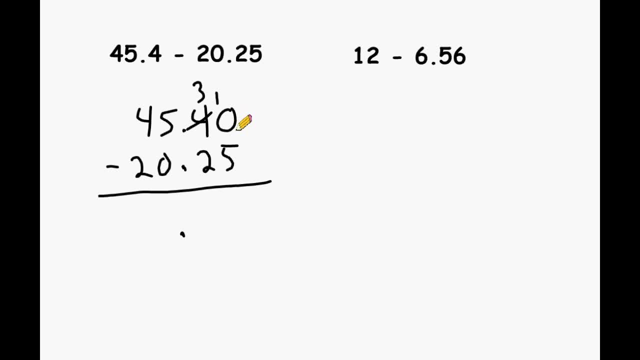 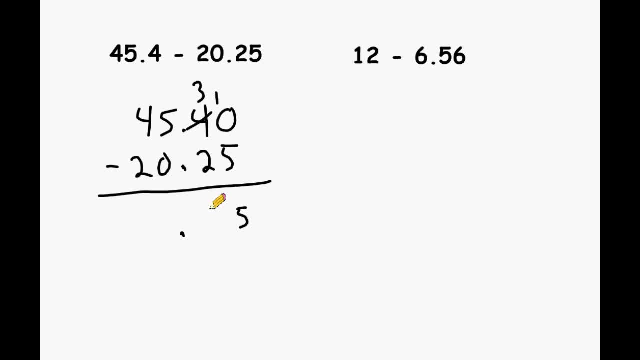 is 5 which is 5 and 3 take away 2 is 1 5 take away 0 is 5 and in this column we have a difference of 2 so the difference of the two given numbers is 25 and 15 hundredths and one last example we have 12 and right away I'm going to write 12 point 0 0 because I noticed with the second number 6 and 56 hundredths we have two place values after our decimal we have to subtract 6 and 56 hundredths from 12 so first I'm going to drop the decimal straight down and then I'm going to perform any necessary borrowing up at the top we cannot take 6 away from 0 so we must turn that 0 into a 10 but we have nothing right next door to borrow from so we have to turn that 0 also into a 10 then we can borrow 1 from that 10 and turn it into a 9 but when we change that 0 into a 10 we had to borrow 1 from this 2 so we have 1 remaining but notice we cannot subtract 6 from 1 so now this 1 we have left must turn into an 11 so we borrow 1 from this 1 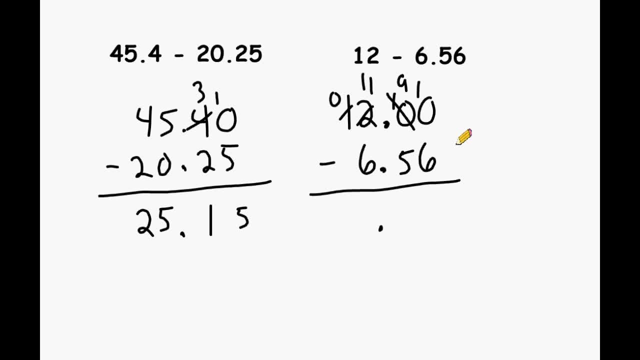 and and that turns into a 0. 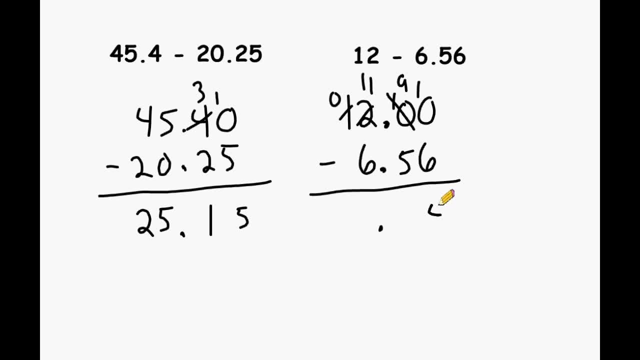 Okay now we can take 6 away from 10 and that leaves us with a difference of 4. In this column we have 9 take away 5, that's a difference of 4 as well. And in this column we have 11 take away 6 and that leaves us with 5. So 12 take away 6 and 56 hundredths is equal to 5 and 44 hundredths. And just to make sure we have the right answer with our subtraction problem it is a good idea to perform the inverse operation. 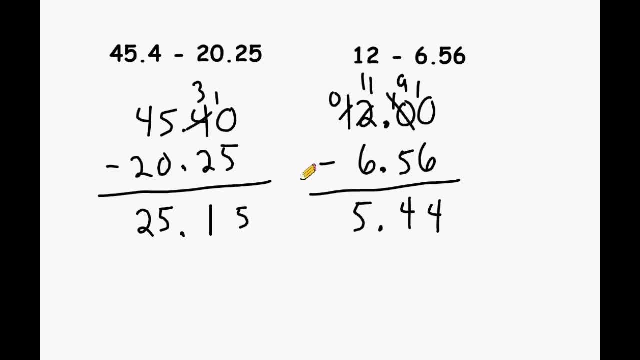 That simply means do the reverse of what you did. Because we subtracted we are going to add to check our answer. So let's take 5 and 44 hundredths and add that to 6 and 56 hundredths to see if we get what we started with which is 12. So once again we drop our decimal straight down and then we proceed to add the hundreds column and in this column we get a sum of 10, carry the 1. This column we also get a sum of 10. 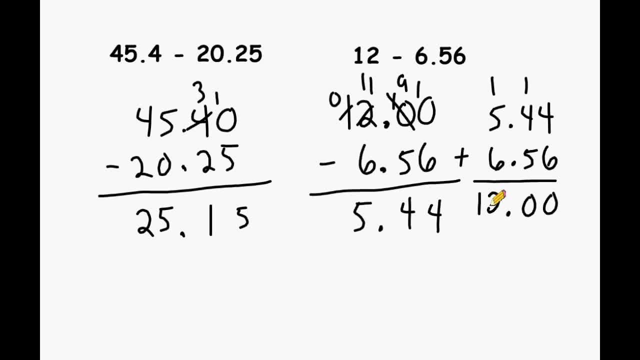 And in this column we get a sum of 12. So by doing the inverse operation we can see that we did in fact perform our subtraction correctly. So we could say that 5 and 44 hundredths is the correct answer. 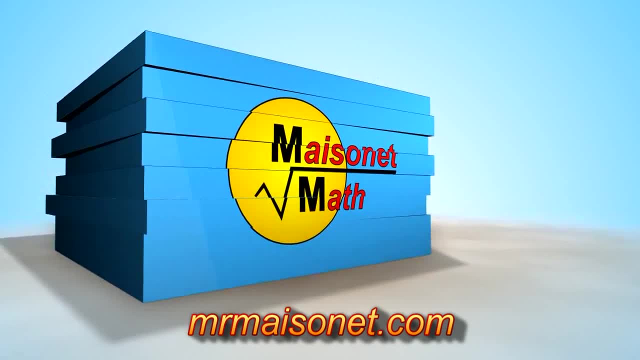 Subtitles by the Amara.org community 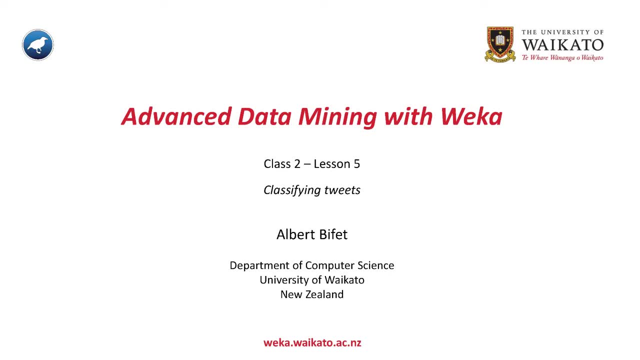 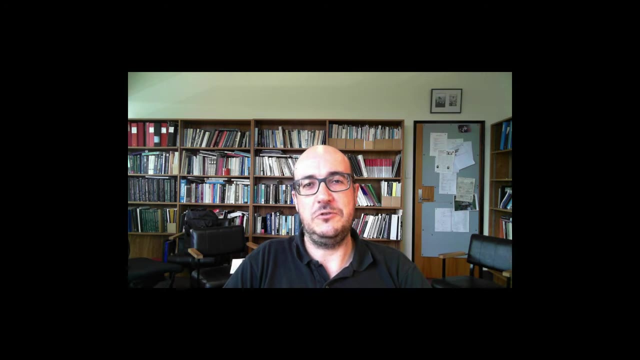 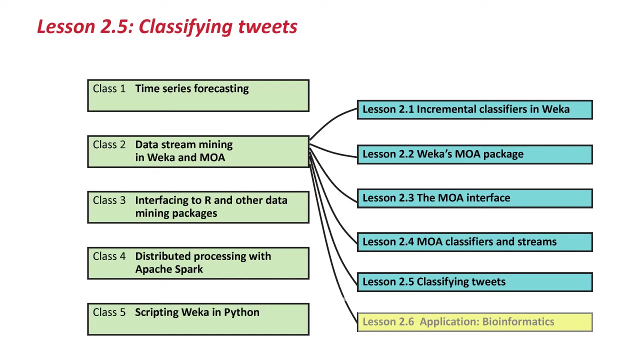 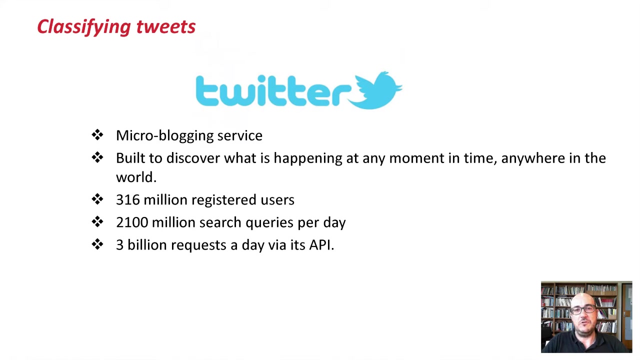 Hello, welcome back to Class 2: Data Stream Mining in Weka and MOA. So we arrived to the last lesson of this class. We are going to look at an application of classifying tweets, So let's start. Twitter is a very nice example of data stream, because it's data that is produced. 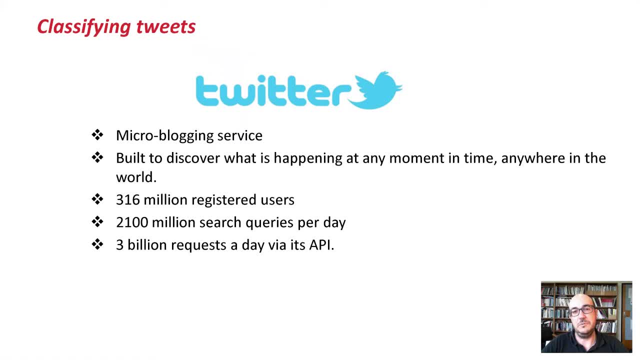 on real time. So Twitter is a microblogging service that is built to discover what is happening at any moment in time. There are more than 300 million users, more than 2,000 million search queries every day, and a very nice thing for us is that data is public and 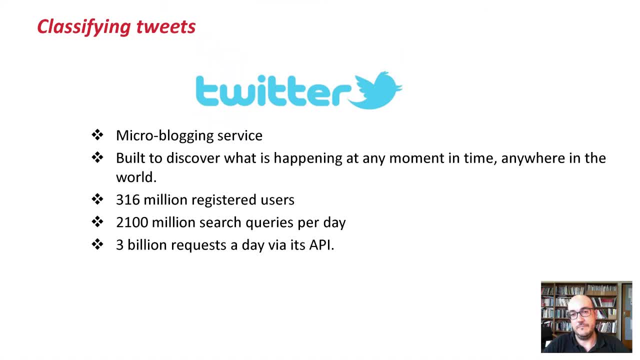 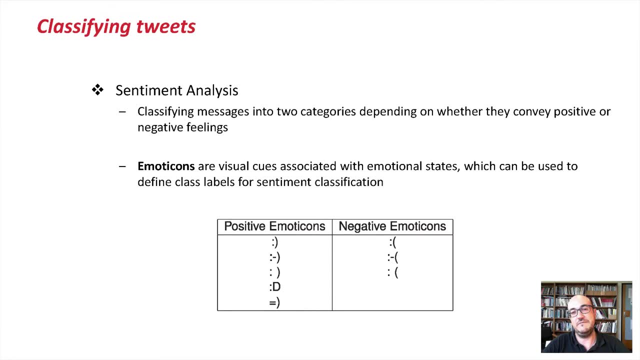 it can be accessed through a streaming API. In this lesson we are going to look at the application of sentiment analysis. So sentiment analysis is the task of classifying messages or tweets into two categories: positive or negative, depending on the feelings that we can see inside the messages. Many times it's 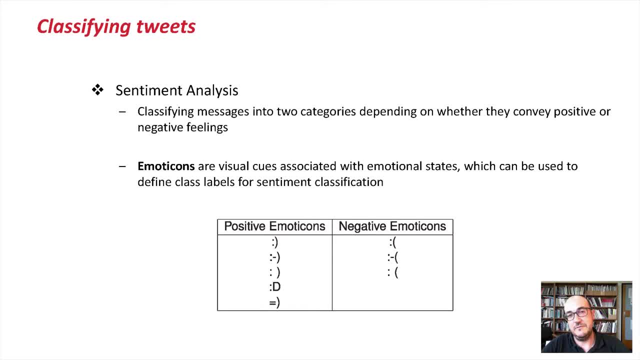 very difficult to get label data In sentiment analysis with Twitter. there is a very basic approach, but it works very well- is that we can get label data using the tweets that they have. So we can get label data using tweets that have positive or negative emoticons inside.